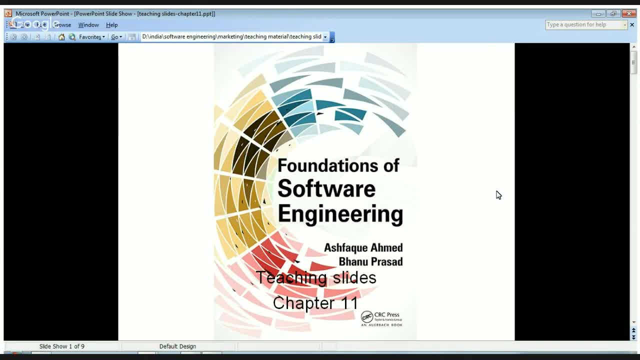 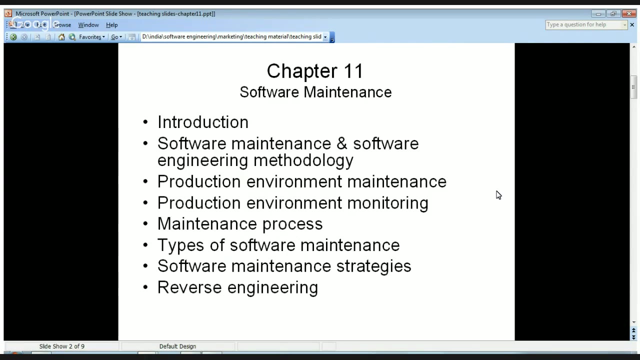 Hello friends, in today's lecture we will see how software maintenance is done. So let us see what we will cover today: An introduction on software maintenance, then software maintenance and software engineering methodology, then production environment maintenance. production environment monitoring, maintenance, process, types of. 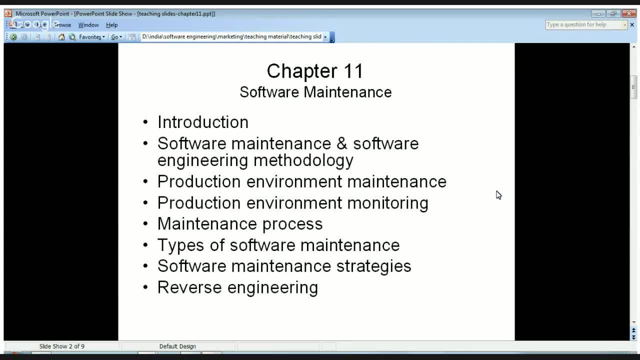 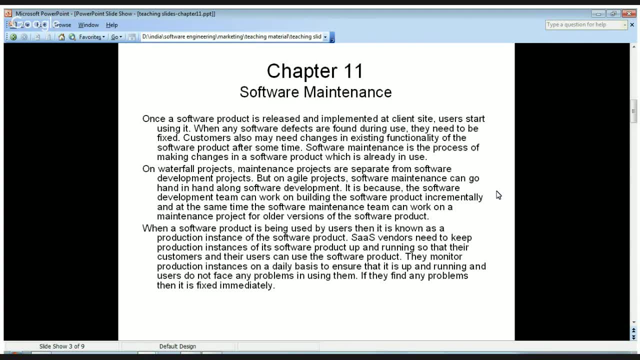 software maintenance, software maintenance strategies and reverse engineering. Once a software product is released and implemented at client-side, users start using it. When any software defects are found during use, they need to be fixed. Customers also may need changes in existing functionality of the software product after some time. Software maintenance is the 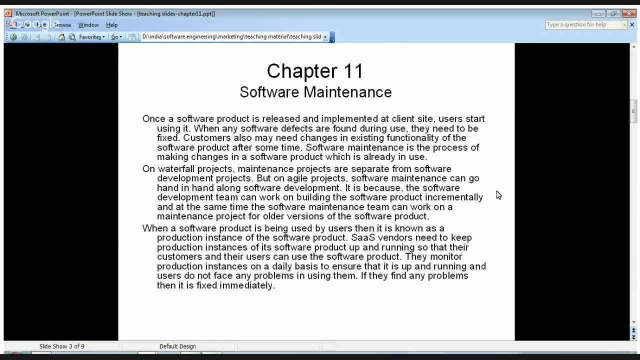 process of making changes in a software product which is already in use. So there is a difference between software maintenance process and software development. In software development a new software product is being developed, So it was never used by any user. But when you do maintenance, 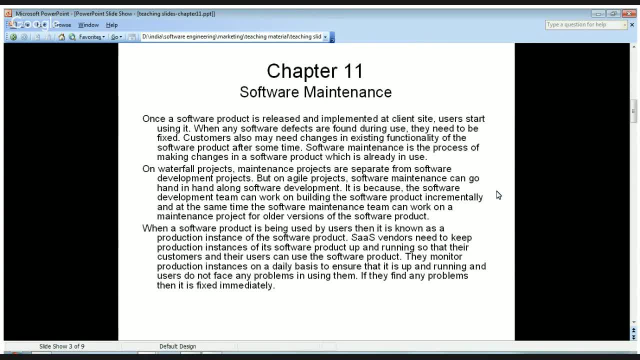 the software was developed and now users have started using it And due to some software defects which need to be fixed or some user request to make some enhancements, you need to take a maintenance project And for this reason software maintenance is done On waterfall projects. 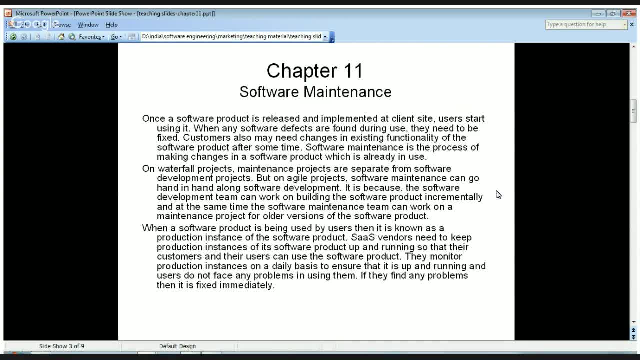 maintenance projects are separate from software development. So maintenance projects are separate from software development. So maintenance projects are separate from software development. So development projects, but on agile projects, software maintenance can go hand in hand along with software development. it is. it is because the software development team can work on building the 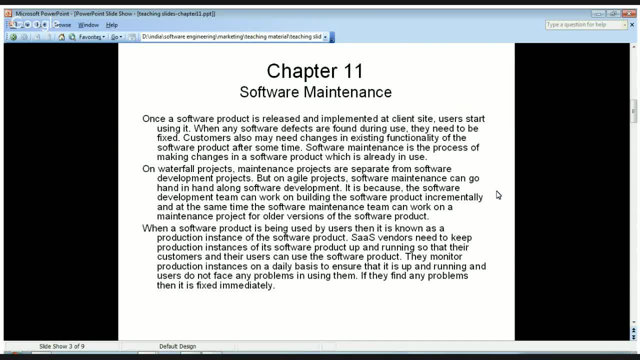 software product incrementally and at the same time the software maintenance team can work on a maintenance project for older versions of the software product. so, uh, there is a difference. when, uh, you have a different kind of projects, like for waterfall projects, the maintenance projects are always separate from software development projects, like first the software software were developed. 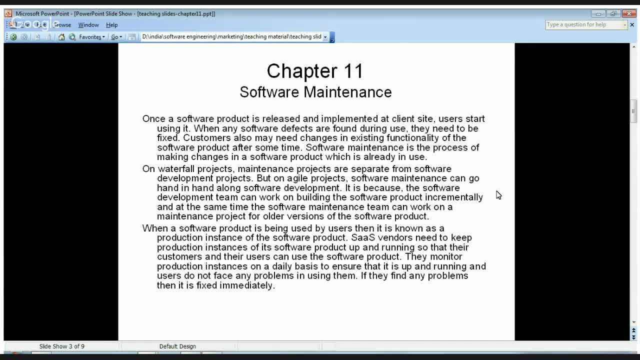 using the software development projects and when the user started using this uh product, then some modern maintenance project can be taken to fix defects or to enhance some features. but in case of agile projects, where the agile model is being used, uh, the software development is happening incrementally. so you already, so this means you have some software product which are 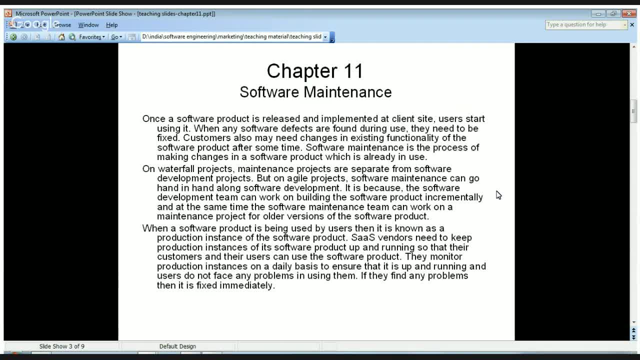 already in use and at the same time some project team is working on working on building new releases of the software product so you maintenance work can be done on the earlier versions of the software and at the same time some software development is taking place for the new release of the software. 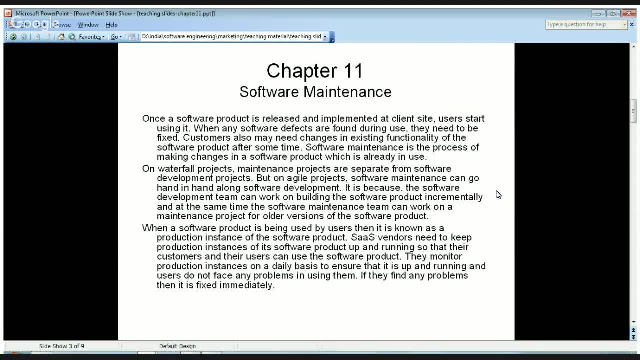 so maintenance work and development work are going in parallel on these kind of projects. when a software product is being used by users, then it is known as a production instance of the software product. so generally the terminology is used as the production instance of a software product when. 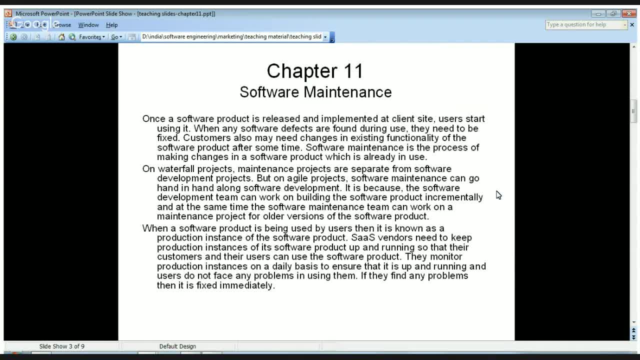 the users are using a version or the release of a software product. SAS vendors need to keep production instances of its software product up and running so that their customers and their users can use the software product. so, in case of SAS vendors, software maintenance is very important and 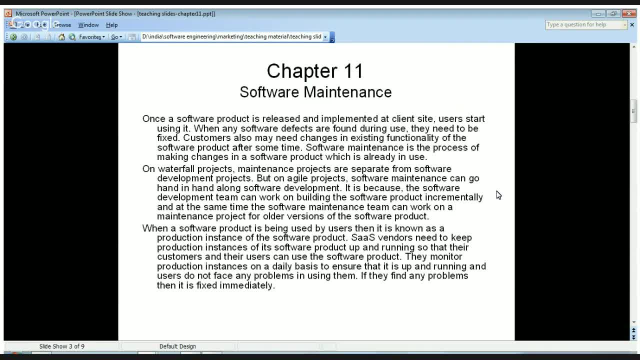 production. running- that means running of their software product- is very important uh because uh SAS vendors get their revenues uh when their customers use their product and pay is for their requirement. like it is a service, the SAS vendor is providing a service to its customers by uh running its software product and the users will be using that software product and they 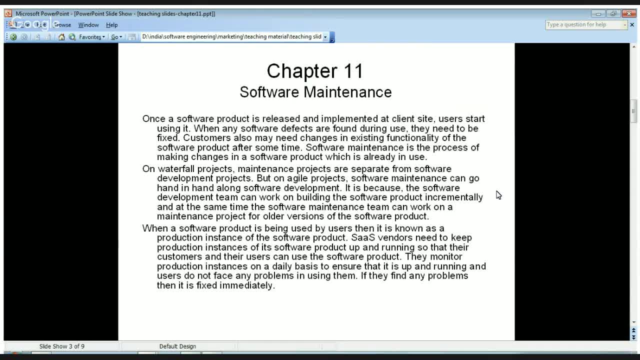 will pay for subscribe service user subscription or something like that. like uh subject: if a customer has 500 users which they will be using a sas product and say per month, the vendor charges 50 dollars for each user, so that means, uh, they will be paying 50 multiplied. 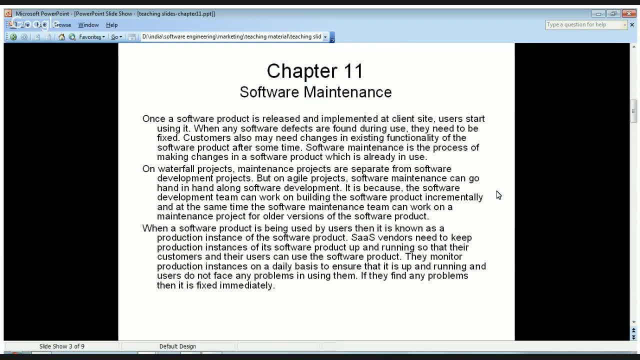 by 500 users per month to the sales vendor. so this is how the sales vendors generate their money. so it is very important that their software product is running smoothly, otherwise the users will not be using and so sas vendor will not get any revenue because the customers are not able to. 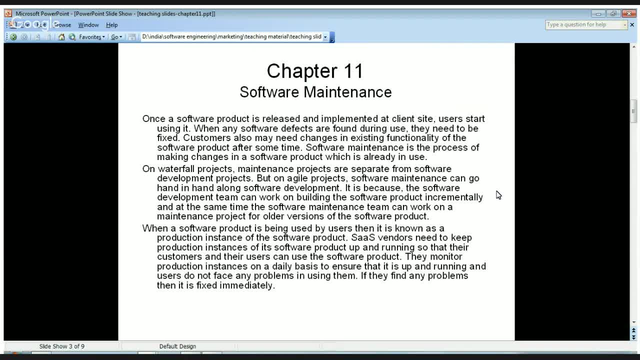 use the software. they monitor production instances on a daily basis to ensure that it is up and running and users do not face any problems in using using them. so the sales vendor themselves monitoring uh the production instances on a daily basis to ensure that the critical functionalities of the software are running fine and if there are any issues, they should be resolved. 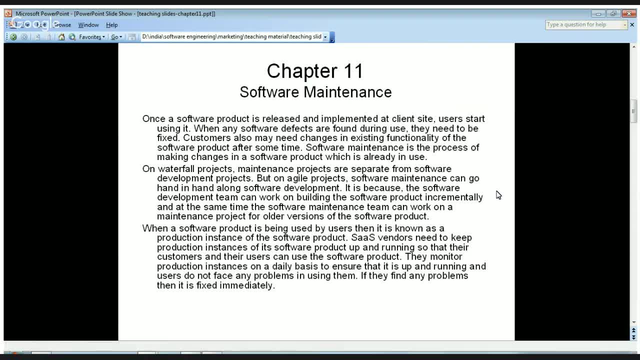 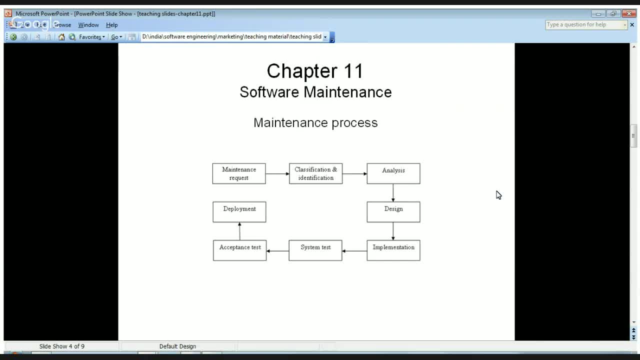 they should be resolved immediately so that users do not get affected due to these problems. and now coming back again to maintenance, so let us see maintenance process. so the maintenance process starts when maintenance requests come from the users. so, based on the request, like what defect or what. 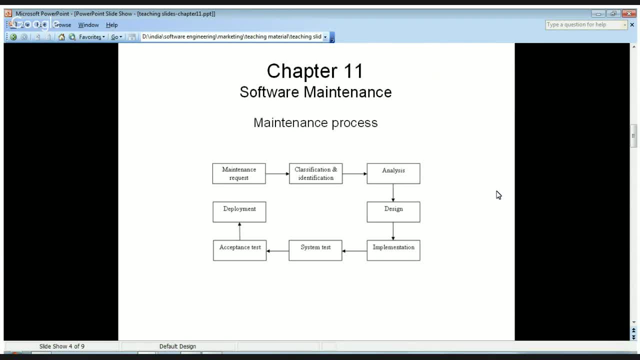 enhancement is required? what effect needs to be fixed? the project team will do classification and identification. they will identify the the parts of the source code which need to be changed. some new source code could be need to be retained in that part of the software product. so they will- and if you they have many- a list of defects or enhance enhancement. 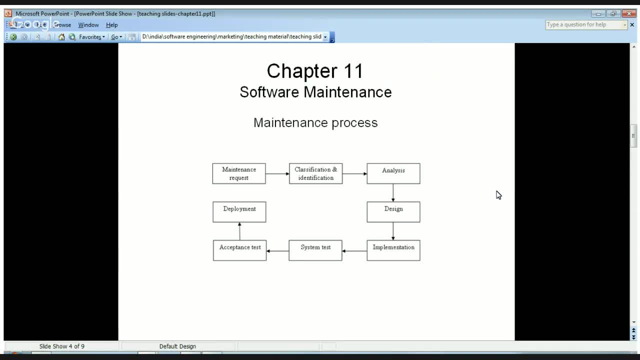 then they will classify all of them, like which are similar and which which have which have more priority, etc. and they will, they will analyze, uh, how the effect has to be fixed or how enhancement has to be done, and based on this they will create a software design. 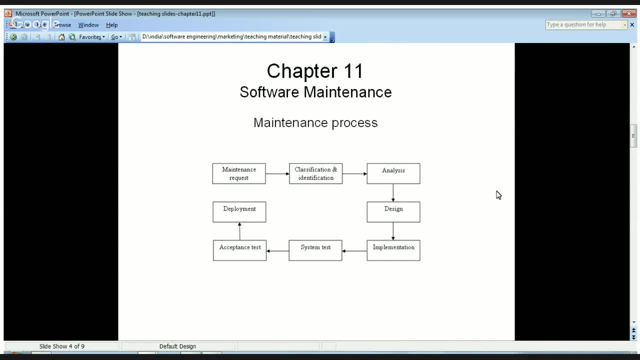 and based on the design. the source code will be retained and the design will be implemented through this source code. and once the software maintenance, like the source code, has been changed or retained, then system testing will be done to ensure that the defects have been fixed or enhancement have been done correctly. 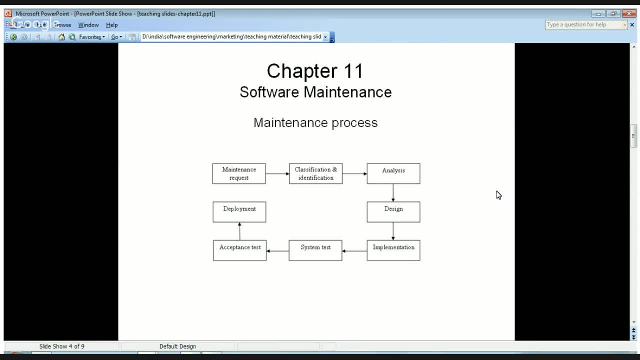 and once system tests are fine, then those changes will be made in the production instance and the users will test means to see if those defects have been removed or enhancement has been done. and finally, this the system will be deployed and used after the tools changing and When a maintenance project is taken to fix software defects or enhance or add software. 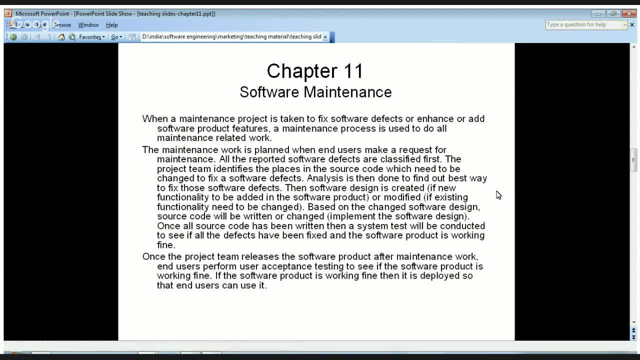 product features. a maintenance process is used to do all maintenance-related work. The maintenance work is planned when the end users make a request for maintenance. All the reported software defects are classified. first, The project team identifies the places in the source code which need to be changed to. 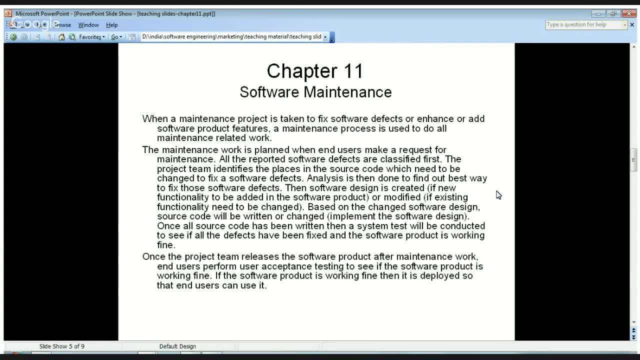 fix a software defect. Analysis is then done to find out best ways to fix those software defects. Then software design is created. if the new functionality to be added in the software product or modified. if existing functionality need to be changed Based on the changed software design, source code will be retained or changed. 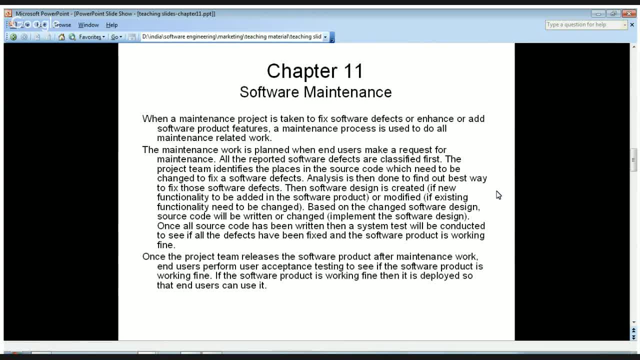 Once all source code has been retained, then a session test will be conducted to see if all the defects have been fixed and the software product is working fine. Once the project team releases the software product after maintenance work, end users perform a user acceptance testing to see if the software product is working fine. 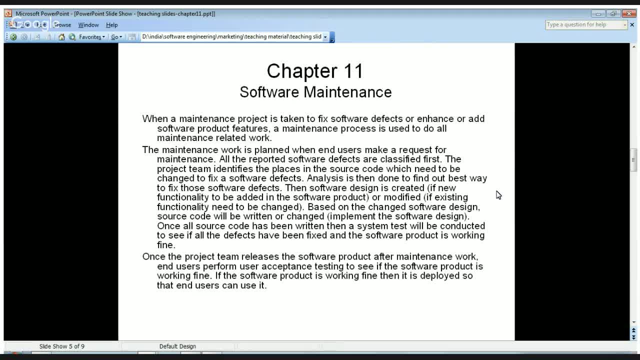 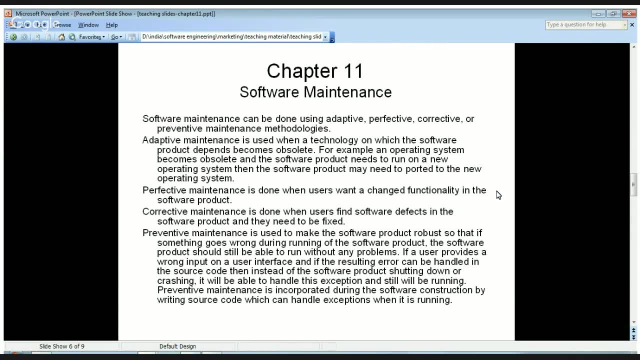 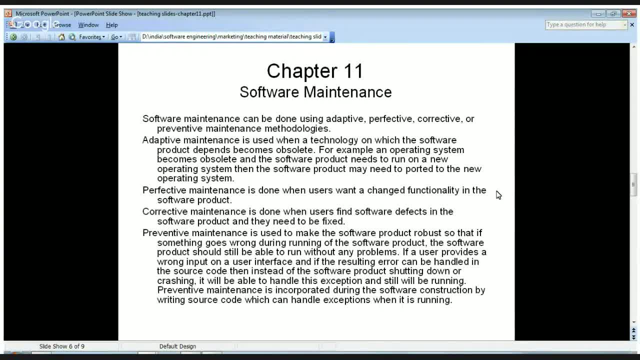 Once the project team is answered for maintenance, their job is completed. Now we have a door on the software product Use a method called TaraSystem. However, Iай nue Canadian텞kngu inform that TaraStasMaitra and Satecp 2050 is working. 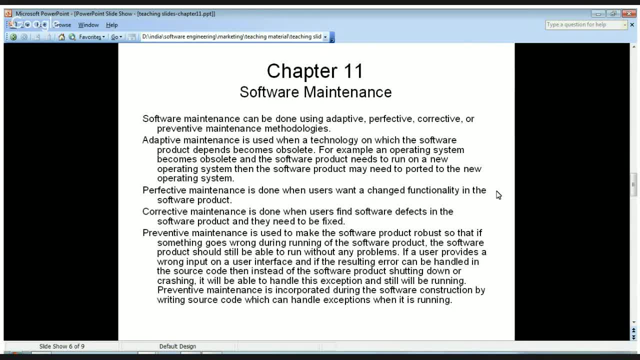 best. this porting of the product on a new operating system is the source code need to be changed so that it can run on the new operating system and for this you need to do maintenance. so this maintenance is known as adaptive maintenance. then we have perfective maintenance and it is done when users 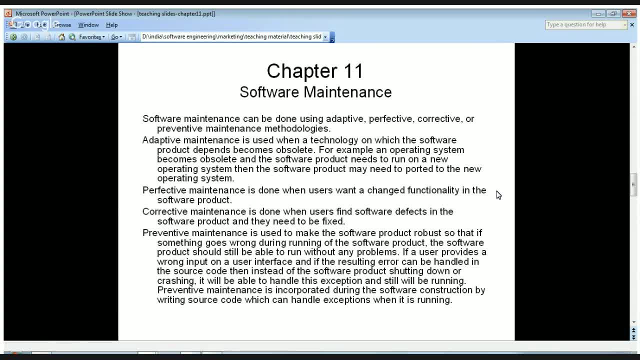 want to change. you want a change, functionality in the software product, so perfective maintenance is like there is a transaction for involving five steps and the users want that. they do not want to go through these five user interfaces where they need to complete the transaction. instead, they want the. 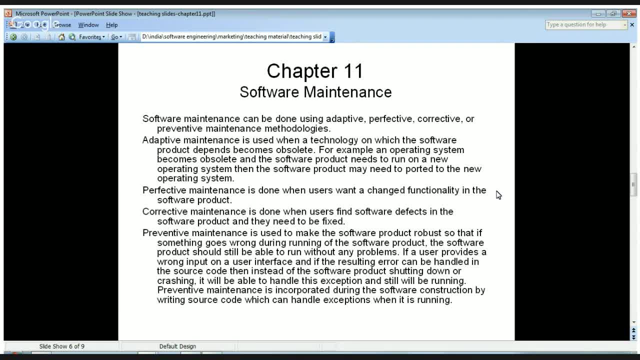 transaction to be done in only three steps and using only three user interfaces. so in that case the software product need to be changed, the source code need to be changed, and so maintenance is required. so in this case it is perfective maintenance. then you can have corrective maintenance where it is done when users 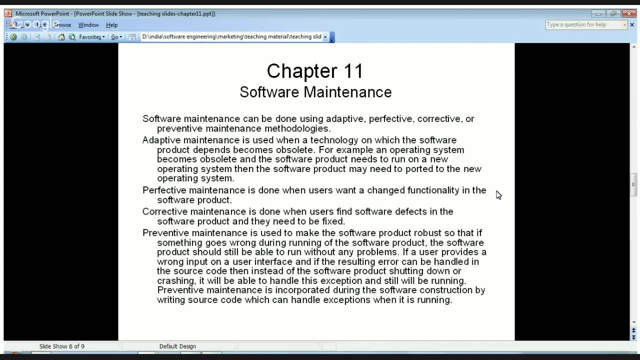 find software defects in the software product and they need to be fixed. so corrective maintenance is done when there are defects in the software product and they need to be fixed. then we can have empty maintenance maintenance and it is used to make the software product robust so that if something goes wrong. 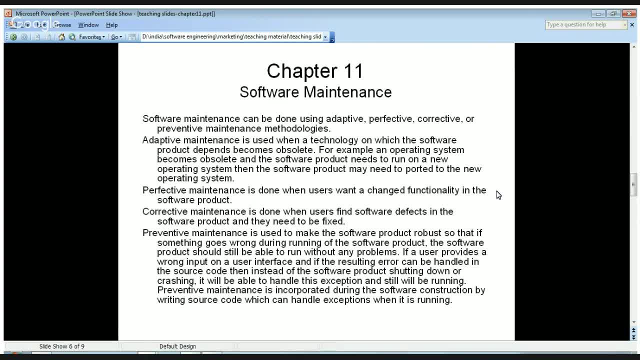 during running of the software product. the software product should still be able to run without any problems. If a user provides a wrong input on a user interface and if the resulting error can be handled in the source code, then instead of the software product shutting down or crashing, 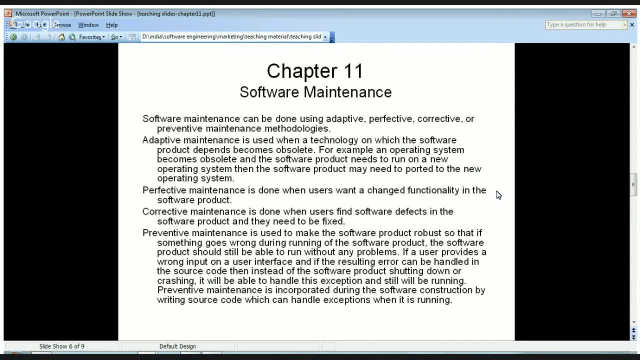 it will be able to handle this exception and still will be running. Preventive maintenance is incorporated during the software construction by writing source code which can handle exceptions when it is running. So you can say: preventive maintenance involves writing source code where the exceptions which can occur during running of the software product can be handled. 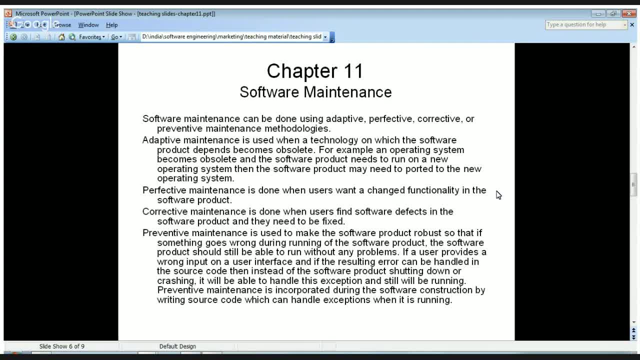 During software development itself. This kind of work is done like, say, you want to do some database operation and so that a database connection is required. So first you need to connect the database and do the database operation. But suppose the database connection is not available or disconnects. 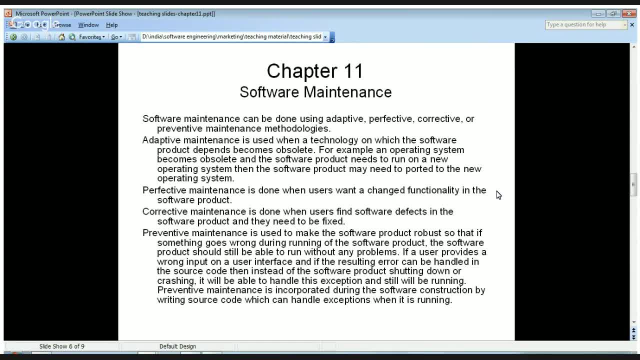 In that case what can happen? like it was connected and some database operation Just started and then some disconnection happened with the database. In that case, what can happen? So the running of the source code or running of the software actually will result in some. 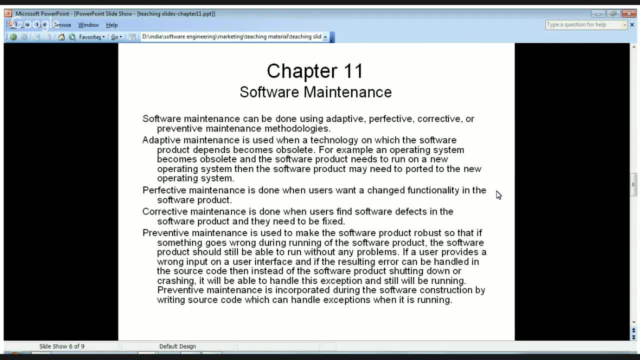 exceptions like the database connection has been reset, So this exception you can handle in the source code itself. Like you can write some routine Where You can handle this exception. like if the database connection has been reset, So you want to roll back all the changes in the database which was happening. so so so that 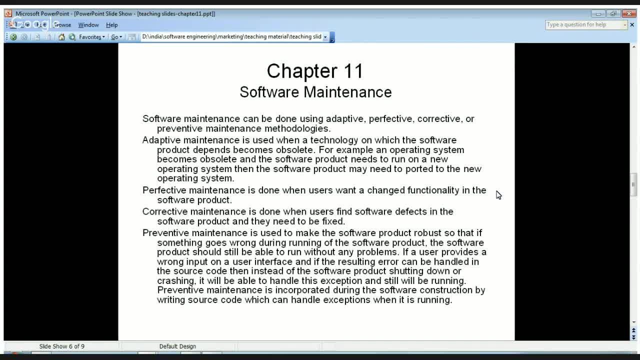 there are no inconsistencies in the database at any point in time. So something like that you can do. similarly, like if the user, the input user, is voiding some input which you do not want, Like, say, you want a password length, the field of the password, field length you want to keep. 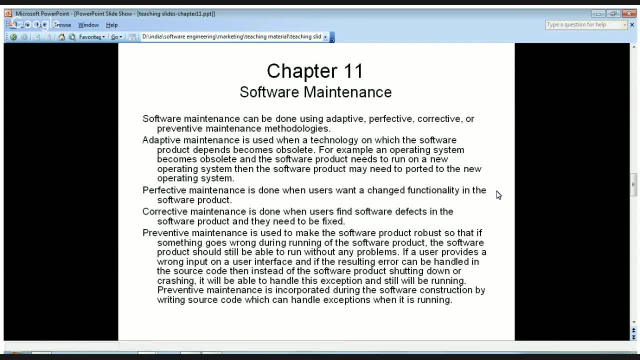 from 8 characters to 12 characters. So in the source code itself, if the user is providing a password which may be less than 8 characters Or more than 8 characters, so you can, you can provide some message box to the user so that 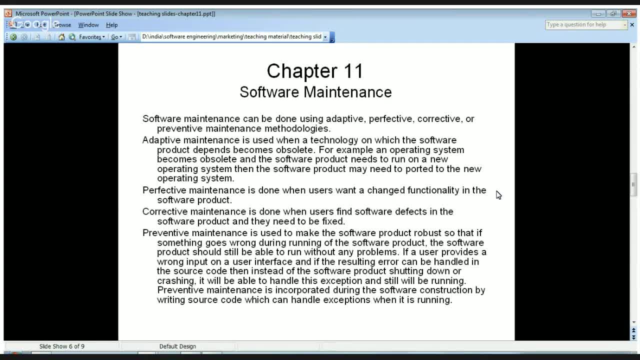 the user can understand that only password can be 8 to 12 characters. So these things you can do in the when you write the source code. So a lot of exceptions happen during development, during running of a software product, Like in doing a transaction. suppose the user has performed a step wrongly. 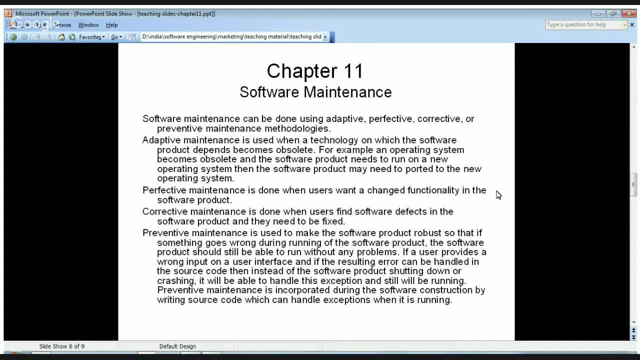 Like he, the user skipped one step and moved to the next step without performing the last step. In that case, the transaction will be faulty. So in that case you can. you can handle this exception And you can write some source code which will allow the user to go back. 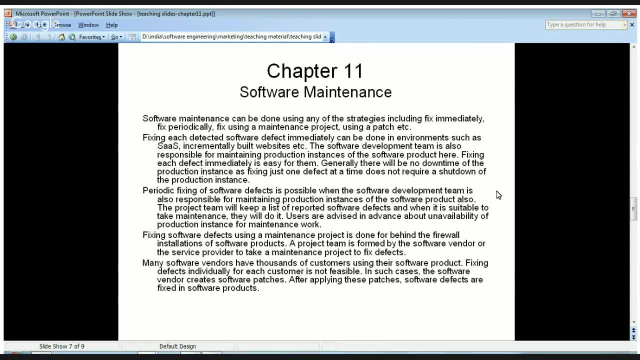 Software maintenance can be done using any of the strategies, including fix immediately, fix, periodically fix, using a maintenance project, using a patch, etc. So software maintenance. there are many strategies for doing software maintenance, So some of them include Fixing immediately, like if a software defect had been found and reported by a user. 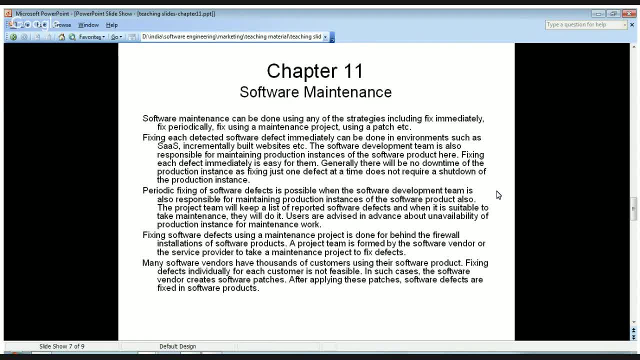 So it can be fixed immediately by the development team And then you can have fixed periodically like the project team will fix, say once per week or once per month, something like that. Then fix using a maintenance project In this case means they will not do any maintenance. 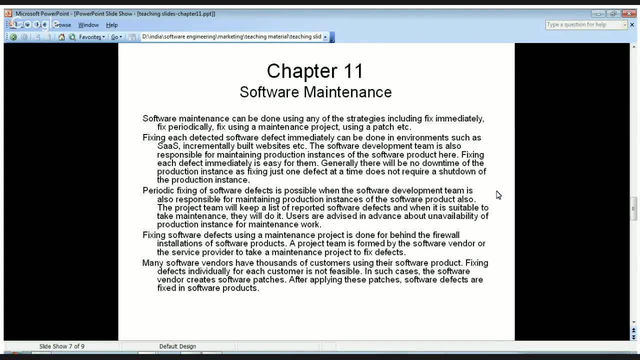 Unless there is a project to maintenance, project is constituted And all the defects will be fixed in that maintenance project. Or sometimes a patch can be used Like patch is, like you know from Microsoft or some other software vendor, The development team for any of the products. 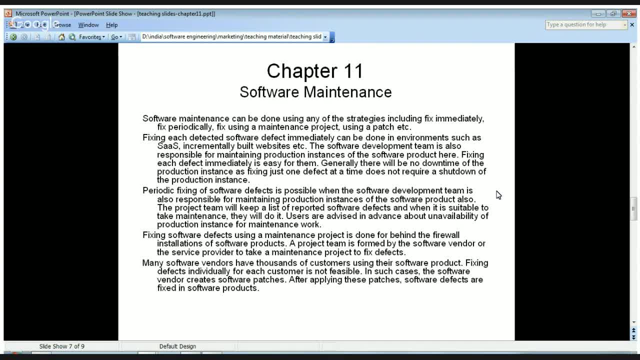 Like software maintenance, The products like, say, Microsoft Word. If it has some defect and users reported this defect, Then the project team will find out the way to fix it. They will fix, And this fixing will be done in a piece of code which can be applied on an already installed product. 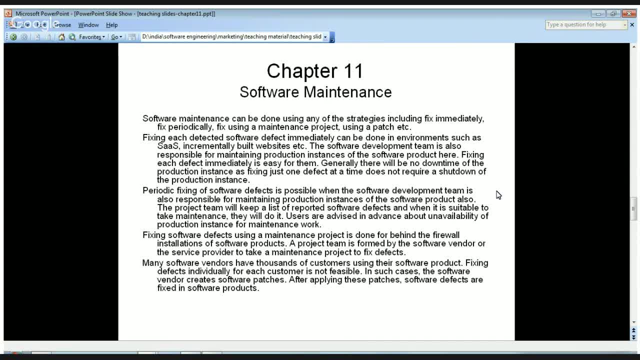 Like, the vendor, will inform the customers that a patch is available for this Microsoft Word product. They can download from their website And you can run this patch so that the existing defect in Microsoft Word can be fixed. So this is how a patch works. 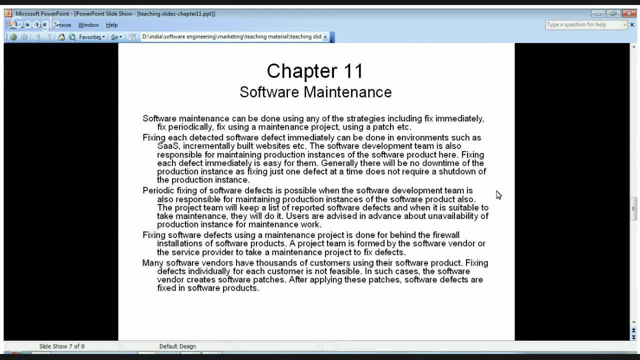 So when you can use a patch, When you can use these kind of strategies for maintenance, So fix immediately can be used for in cases where you have a fast product Or you can have a incremental development team. So you have already released version of the software product. 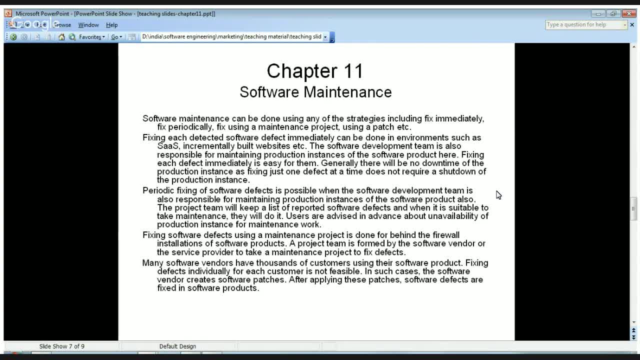 And the product development team is there. So the product development team is working on building some new releases And in that case, since the project team is available, Which has been working on the same product, May be different releases, So it is possible for them to fix it immediately. 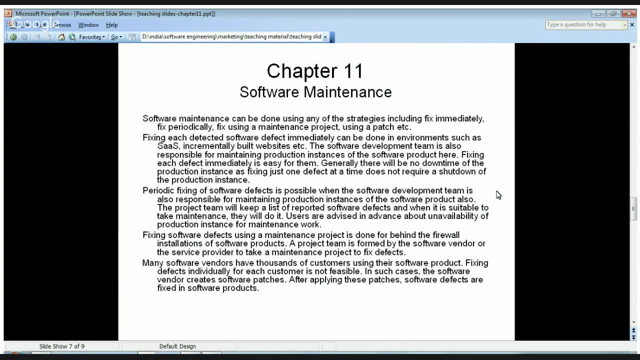 So it is suitable in that scenario. Then fix periodically. So fix periodically means the project team is busy in doing something- In this scenario like working on incremental development- But they are busy, They do not have time to work on any defect. In that case, what they can do: 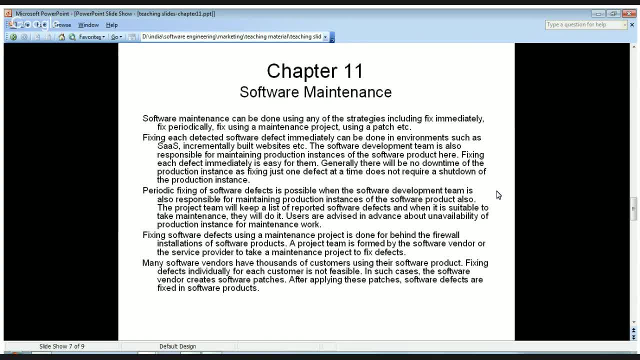 They can fix a time, Say once in a week All the defects which have been reported They will fix on that is a sick date. So this scenario Can be used in that kind of working condition. Then in some cases maintenance project is required. 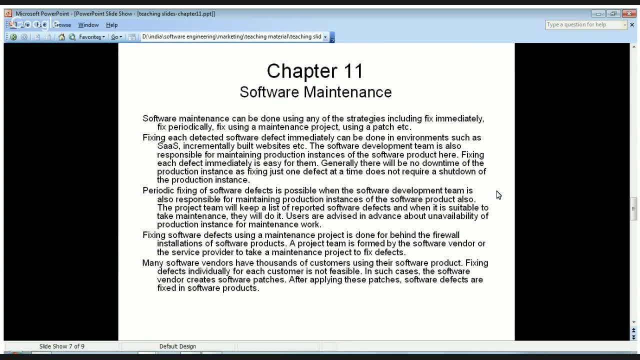 So generally maintenance project is required For products which were built using waterfall model. So after building of the product The project team was disbanded. Now there is no project team Which is working on that software product, So in that case if the users found defects in the product, 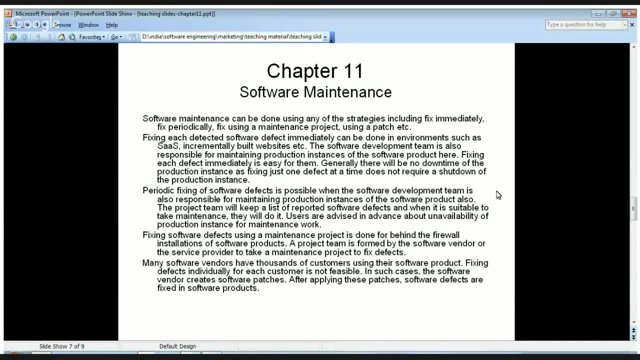 In that case the vendor or any service provider Can be asked to take a maintenance project for that product. In that case project team will be built for doing that maintenance. Then patch Patches are used in the scenario I had given before. 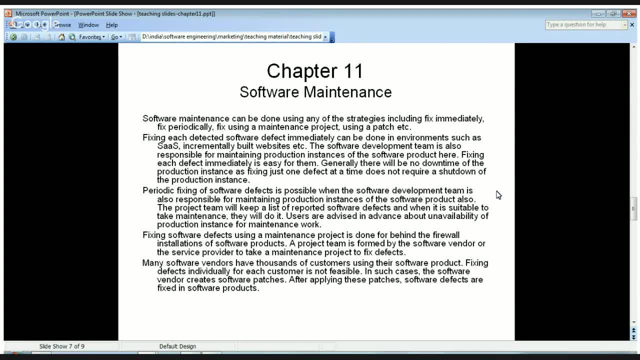 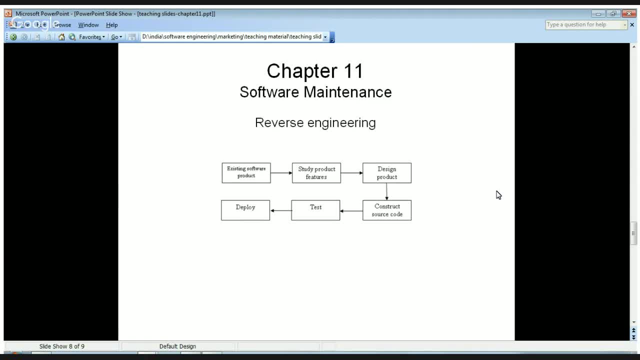 Like for software vendors, It is possible to create patches To solve any problems due to defects. Now let us come to understand reverse engineering. Reverse engineering is one of the methods Where, suppose, you have a software product Which you are using And you only have the executable binary code? 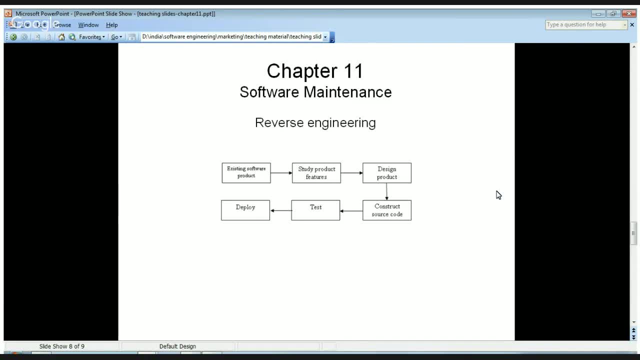 And this software product Is now no longer being supported by the software vendor, So nobody who have the source code of this product And, at the same time, You found that there were some defects And you want to Make this product useful. 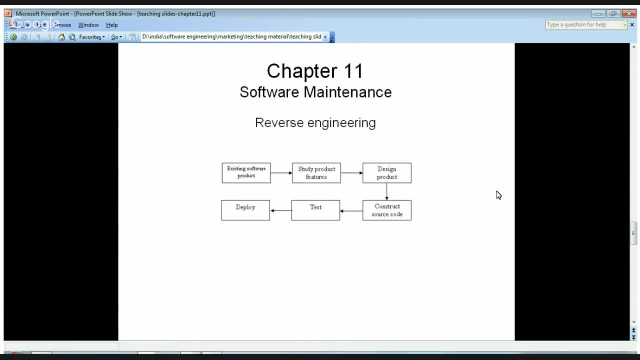 And you want this product to be used by your users. So in that case, what options you have? Because it is not supported anymore by the vendor And nobody can fix those defects. In that case, what you can do is You can use reverse engineering. 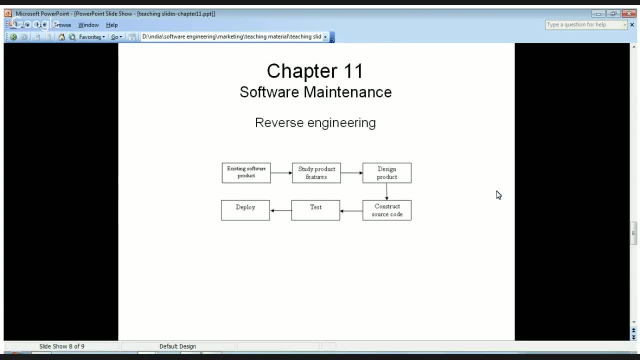 To find out the design Of this software product, And then you can build a software product Which is very similar to the product you are using, So that your people can use the newly developed software product, Which is almost the same as the old one. 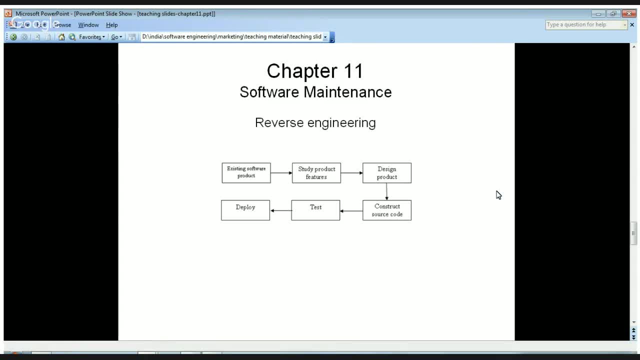 But the defects which were there in the earlier product Are fixed in this new one. So this is known as reverse engineering, Because you are going back To find out the design of a software product. So this is known as reverse engineering. So this is how you use it.